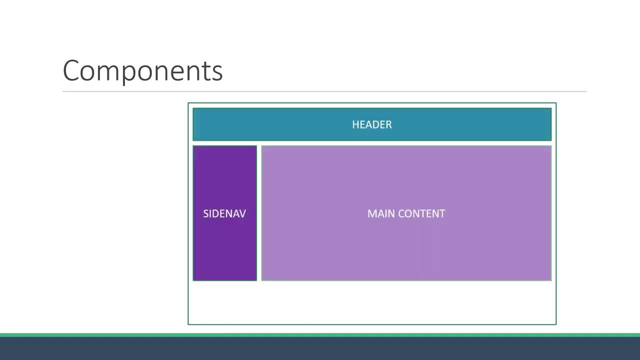 down into header, side nav, main content and footer. You can say that this particular application has five components: One component for header, one for side nav, one for the main content, one for footer and, finally, one component to contain every other. 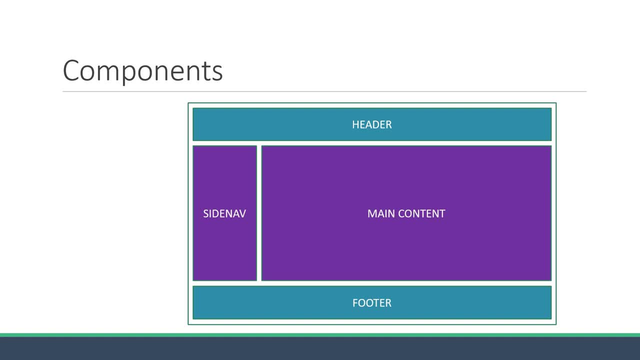 component. The containing component is the root component and is usually named as app component written in a file called appvue in your project. Each of the four nested components describe only one component. The component that contains the component is called the root component. This is only a portion of the UI, However. all the components come together to make up the entire. 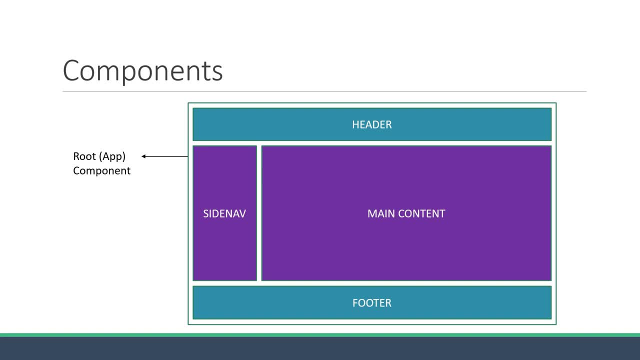 application. The components are also reusable. The same component can be used with different properties to display different information. For example, the side nav component can be left side nav as well as the right side nav. Only the data has to change. Now, how does a component 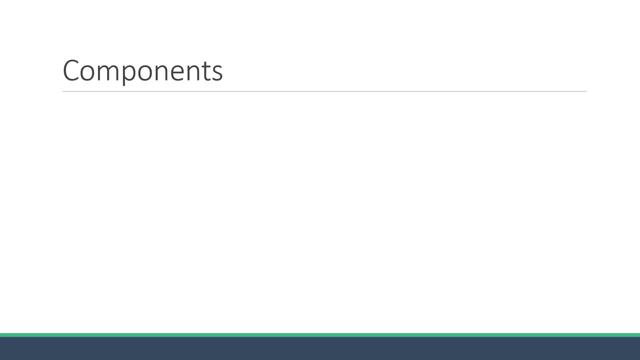 translate to code in our application. Well, we have seen that bit quite a lot. A component code is usually placed in a vue file and can contain a template block, a script block and a style block. appvue is one such example, But in a real-world application you're often going to create 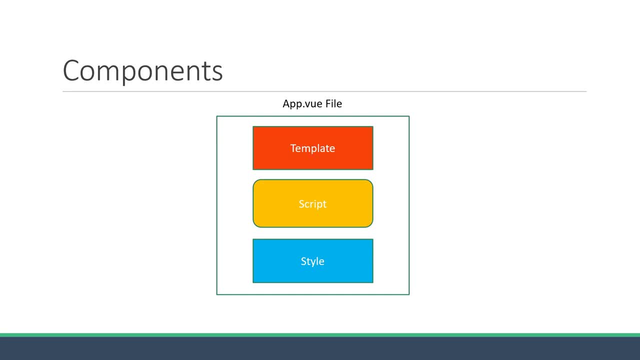 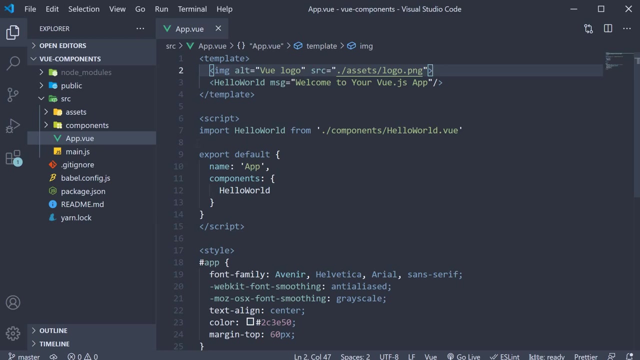 tens or hundreds of components, each describing a portion of the UI. In this video, let's learn how to create and register a new component in our Vue application. To get us started, I have created a brand new project to learn all about components in Vue. 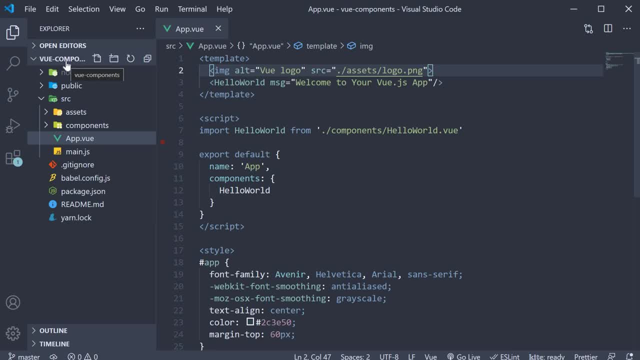 The project name is Vue-Components. You can find the same on my GitHub repo. We want to start from scratch, but the CLI does generate the hello world component for us, which we don't really need for this video. So let me delete the file and the code pertaining to the hello world component in appvue. 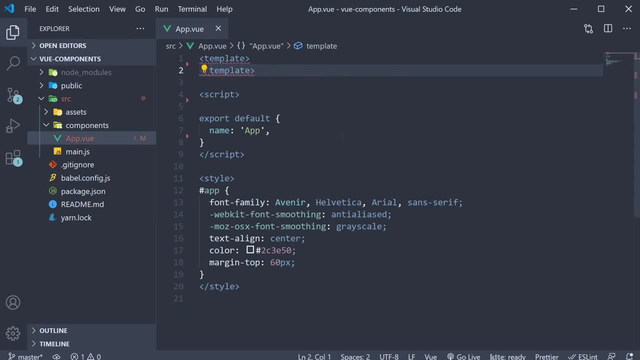 Let me also remove the logo. Alright, now let's create our very first component in Vue. The component will simply output a message: hello Vishwas. in the browser. In the components folder, which is automatic, let's create a new file called greetvue. 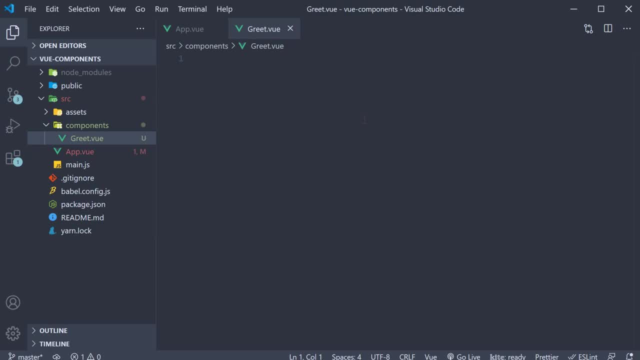 This component needs to render the text hello Vishwas, So we definitely need some HTML. To define HTML in a Vue file, we use the template block, So add a template tag, an h2 tag, that says hello Vishwas. Alright, we now have the HTML in our Vue file. Let's create a new file called greetvue. 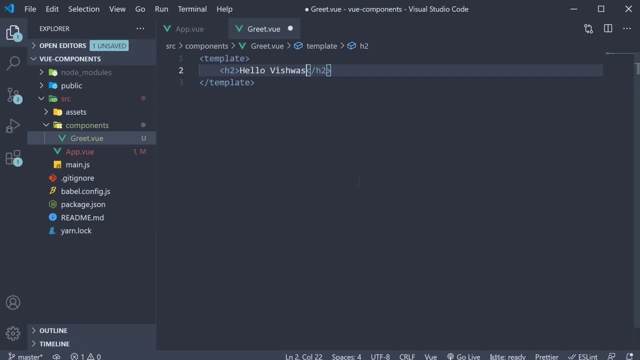 This is the HTML that needs to be rendered in the browser, But as it stands now, the HTML hello Vishwas. is not going to be rendered in the browser, because this greet component is in no way connected with the rest of our application. 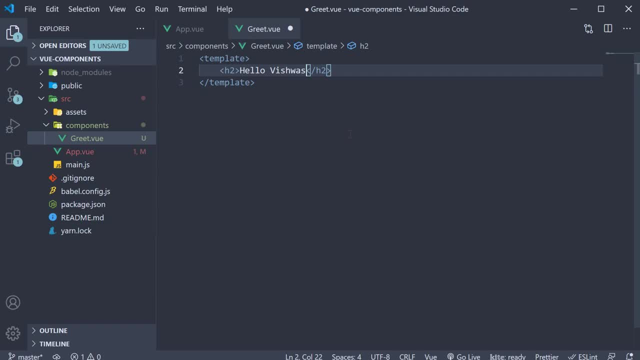 So what we have to do is export this greet component from greetvue, import it in appvue and then include it in the app component template. In other words, we need to register the greet component with our application. Let's start with the greet component export. 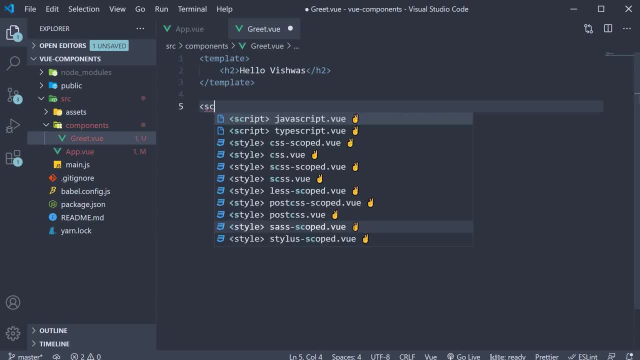 After the template tag, add a script tag. Within the script tag we default export an object. The object contains a property called name, which is pretty much the name of the component. Let's name it greet. Now that we are exporting this component from greetvue, let's import it in appvue. 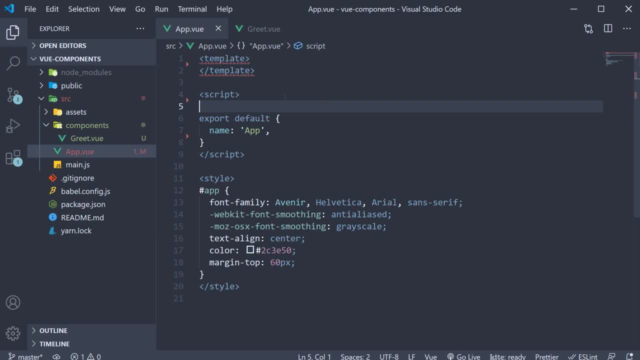 So in the appvue file, within the script block, first import the component. Import greet from dot slash components, slash greetvue, which is the path to the greet component. Now to include the grid component in AppComponent, we specify the component as a custom HTML. 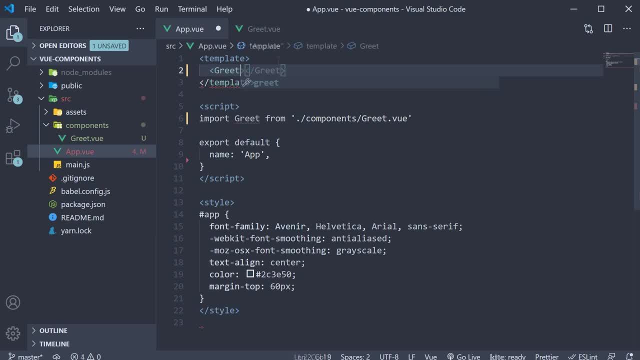 tag in the template block. If there is no content between the tags, we can change it to a self-closing tag. However, AppComponent doesn't recognize the grid component yet In the script block we need to specify a property called components and specify the. 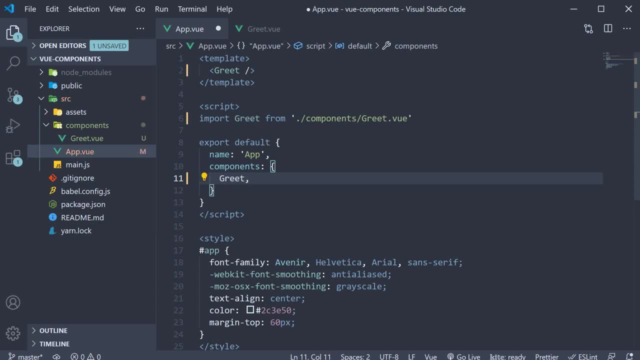 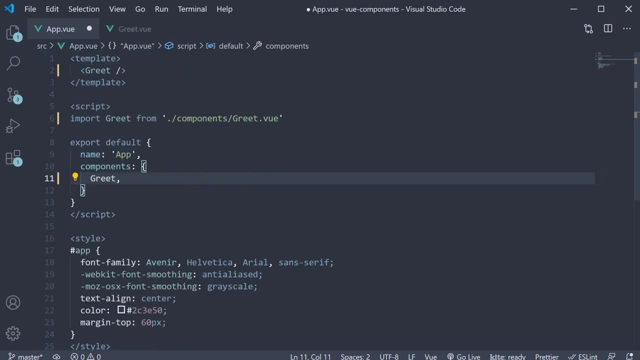 key as well as the value as grid, but we can use the shorthand syntax in ES6, so grid is the key as well as the value. We are basically informing Vue about the grid component to be utilized in the AppComponent. If you now save all the files and take a look at the browser, 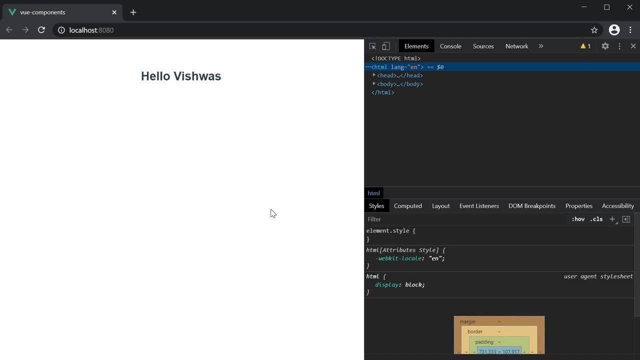 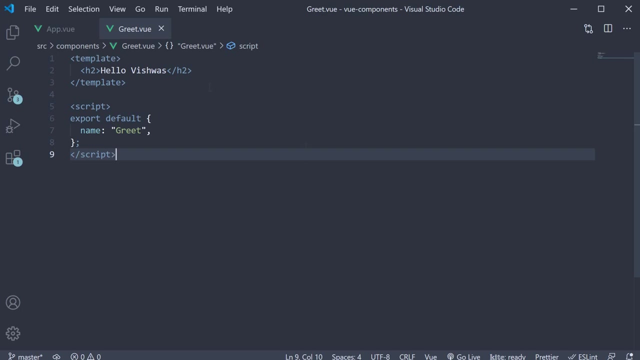 You should be able to see HelloVishwas. Your first Vue component is up and running. Before we proceed, there is one thing I want to highlight. When we create a new component, it is pretty common that you would want a template block. 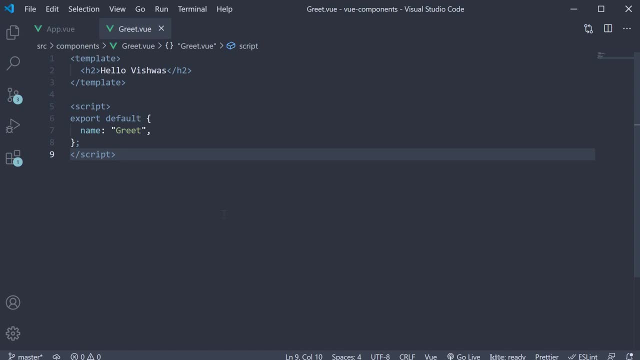 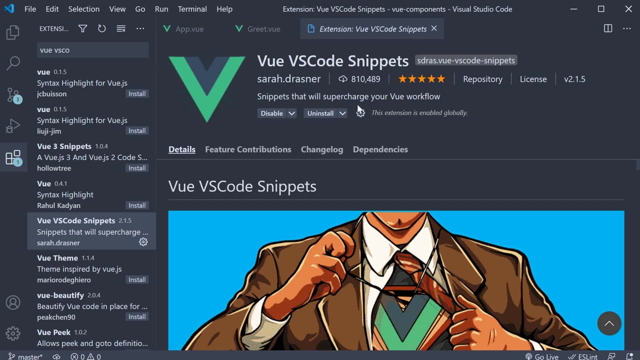 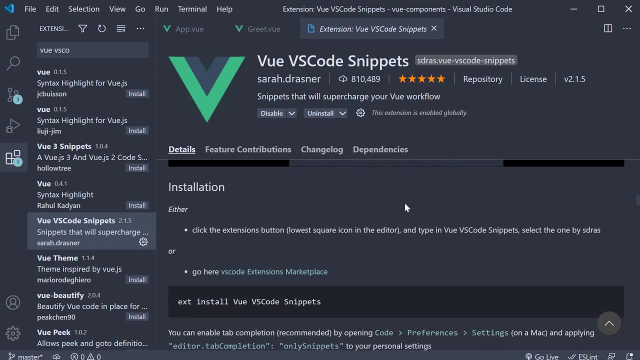 a script block and perhaps even a style block to add some styles. To help you with this, there is a VS Code extension which I recommend you install as well. It is called Vue VS Code Snippets by Sarah Drasner. The extension gives you a lot of code snippets to improve your coding speed, if I can call. 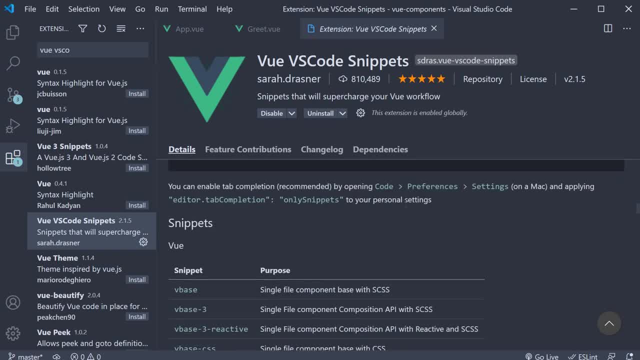 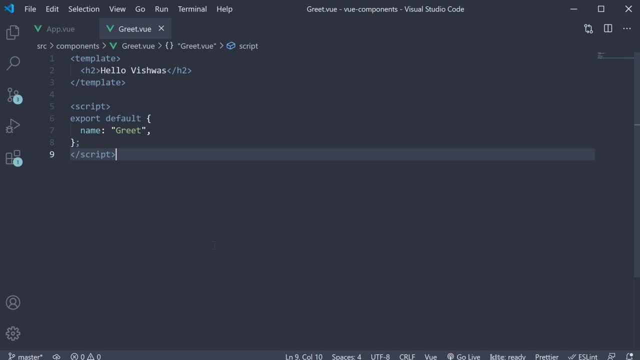 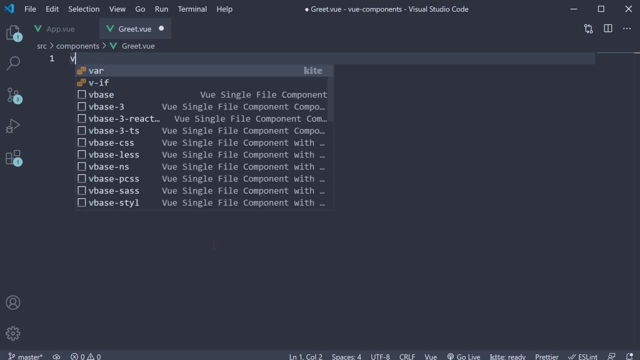 it that, So go ahead and install it. Once you install it, creating a new component is very easy. Let's rewrite the code for the grid component using the Vue Snippet, Clear all the code And then Type vbase-css. 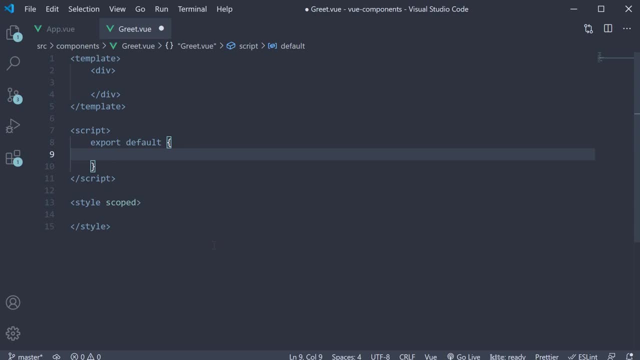 As you can see, it gives us the skeleton code for an entire component. We can now make the necessary changes. Template is an h2 tag with the text HelloVishwas. The default export contains a name property And we also have a style block.